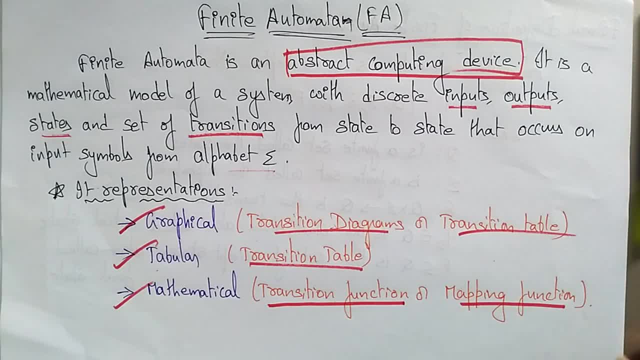 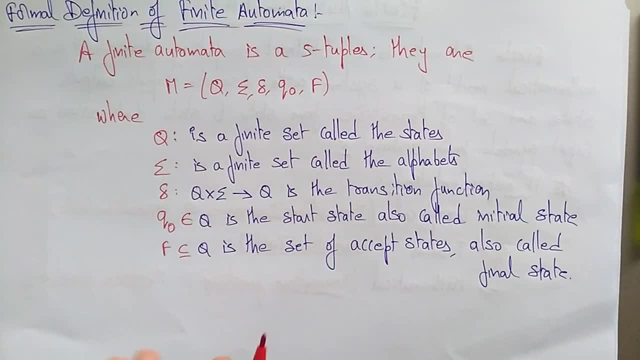 represented either in graphical tabular or transition function. So let me explain you the formal definition. So I said what the finite automata is, consisting of set of tuples, set of inputs, outputs and some things will be there So that you call it as a. 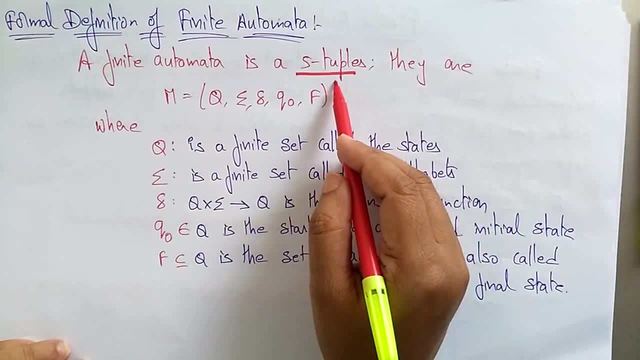 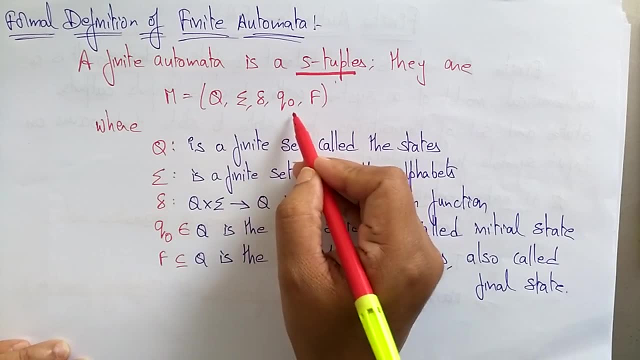 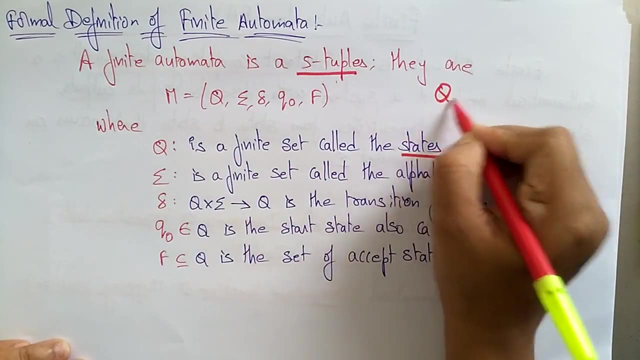 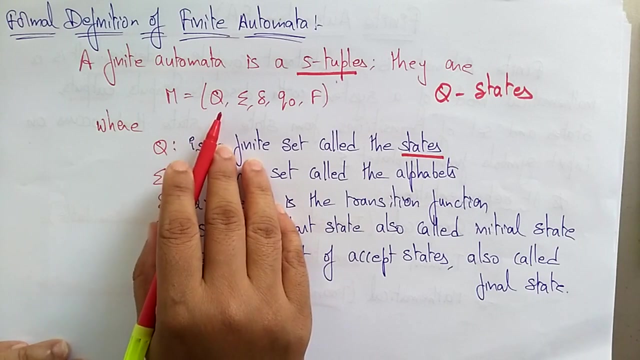 tuples. A finite automata is a phi tuple. There are Q sigma, okay, delta. Q naught F. So here Q, you call it as a finite set called states. So Q represents the states, A, Q in this language you call it as a finite set called the states, And you already know. 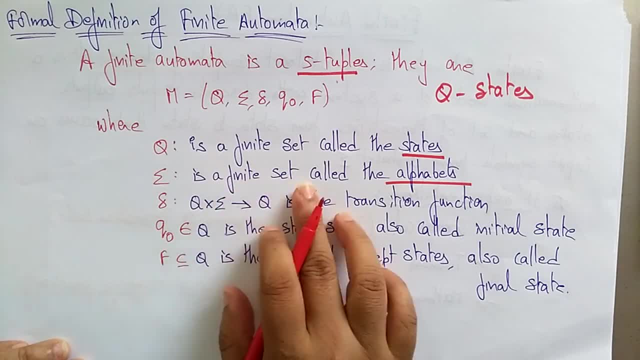 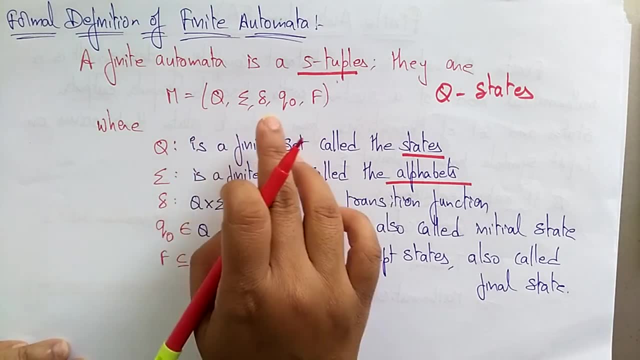 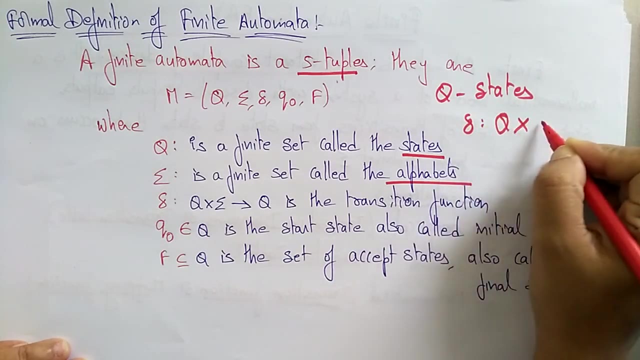 the sigma is nothing but the finite set. It is a finite set called alphabets, Sigma. you already seen Sigma is an alphabet, Q is a set of states And coming to the delta, Delta is nothing but it is a combination of states into alphabets. You will get a Q. 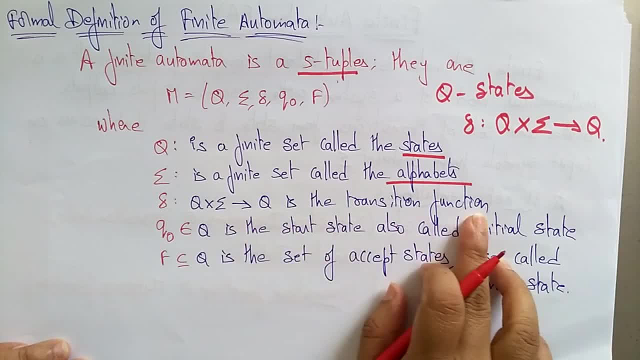 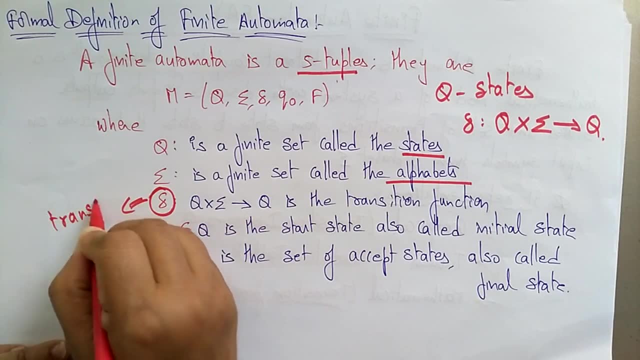 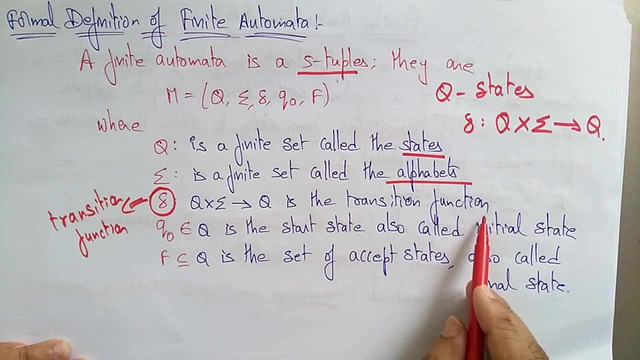 So Q into sigma, else Q is a transition function. So remember that This delta, you call it as a transition function. Q into sigma implies the next state, A state with the finite input state. you will get another state. That is a transition function And this Q naught, you call it as a start. 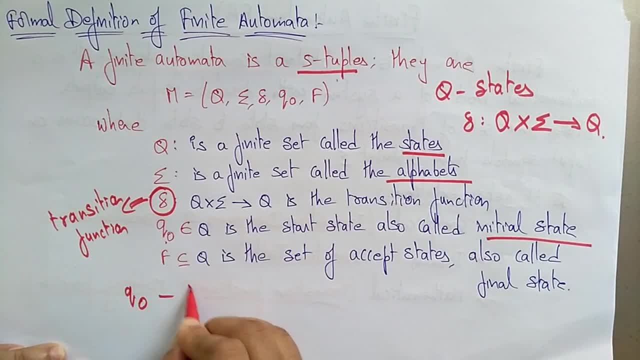 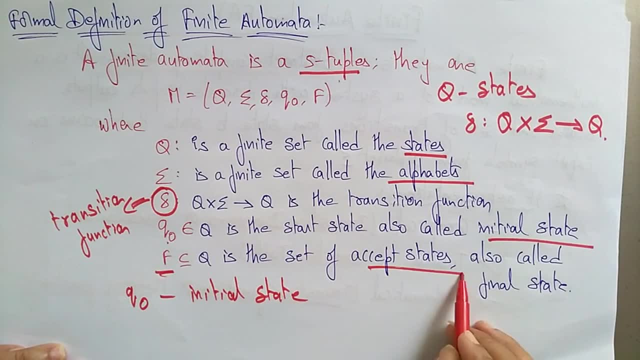 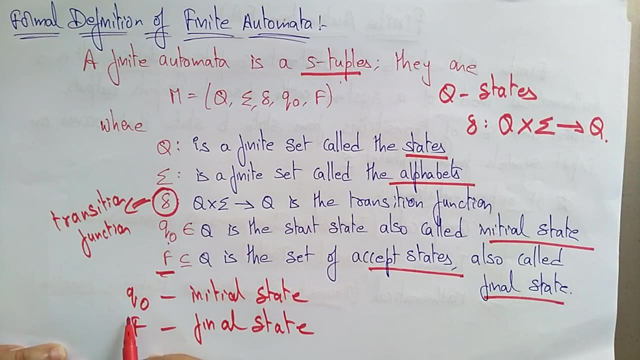 state, also initial, So Q naught is remember that it is initial state. Or also you call it as a start state And F you call it as an acceptance state or final state. F is final state, So starts with the Q naught and 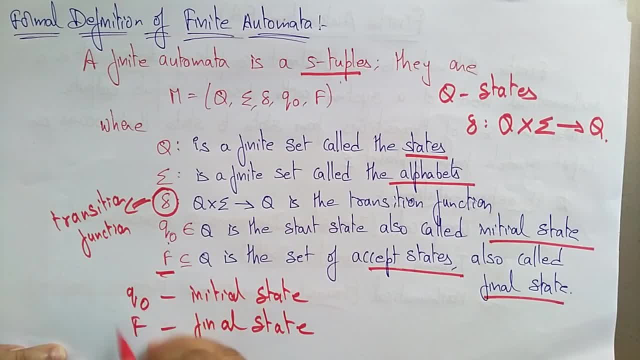 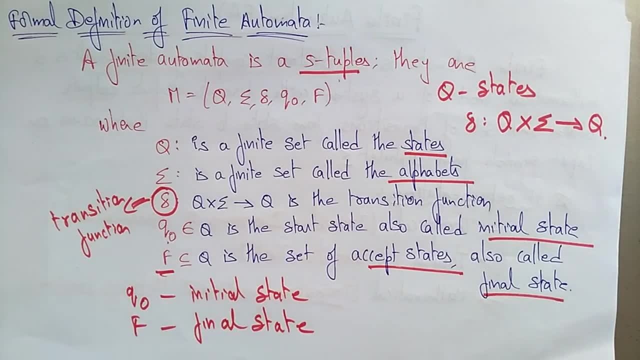 end with the final state, F. So these Q, naught and F will be present in the finite set called the states. These are also called as a states. So remember that The formal definition of finite automata means you have to write this definition. It is just a simple It consisting of five. 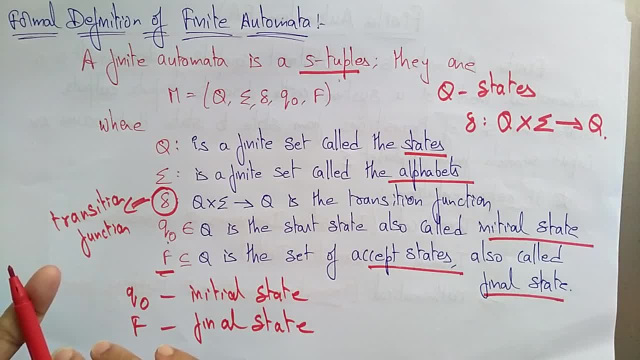 tuples. What is that? Q consisting of finite set states, Sigma is a set of alphabets And delta is a transition function. Q naught is a initial state And F naught is a final state. That is it, A finite.